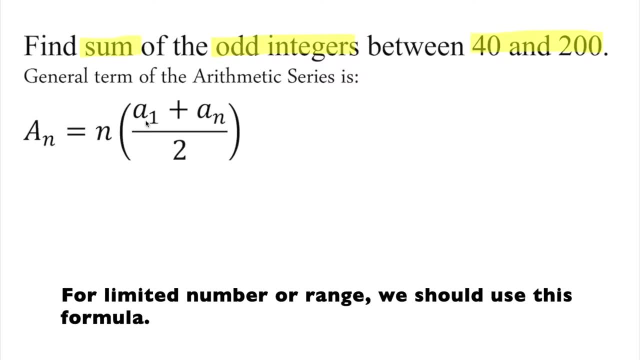 So we're going to figure it out. So unknown values, n, an or a sub 1 or an, But we can find those out right from the problem. the key is given here though. So well, n, Let's go with the n first here. So let's find the n. So n is equal to 200 minus 40. We find the range, and whatever the range. 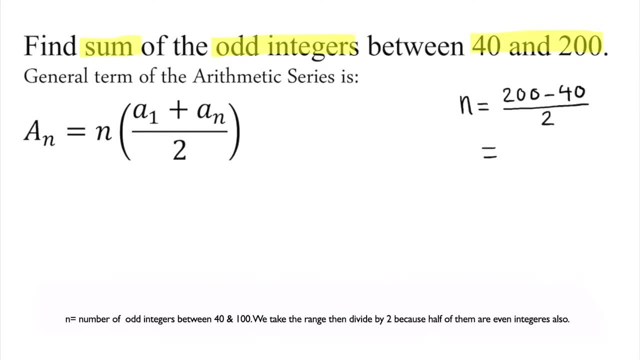 divide by 2.. The reason we divide by 2, is because 160 divided by 2, 160. between this one and this one there is 160 numbers Which numbers Odd numbers. So out of this, half of the number or half of them are even number. But we are looking. 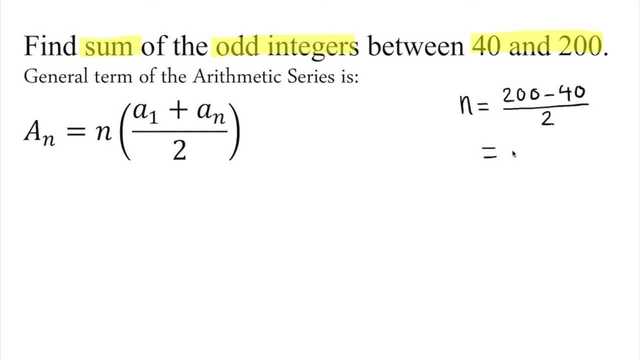 for odd number in this case. So well, what is n? So n is in this case is 160 over 2, which is 80. That is our n. We have n, So the next thing we look for a1.. So that is going to be crucial. 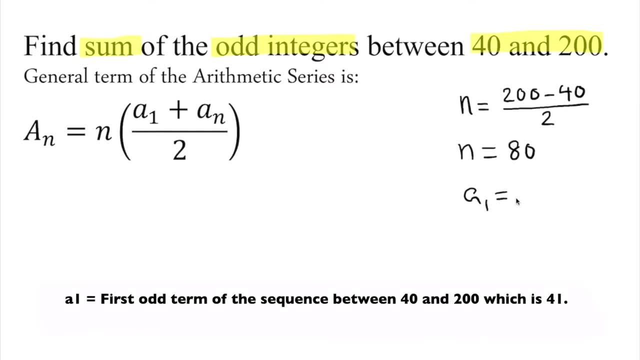 This is going to be very important. So a1 is supposed to be what? 40?? No, not really, a1 is 40 is telling us to look into that condition. What is the condition? Odd, And of course, what is the first odd Right after 40, which is 41. So that 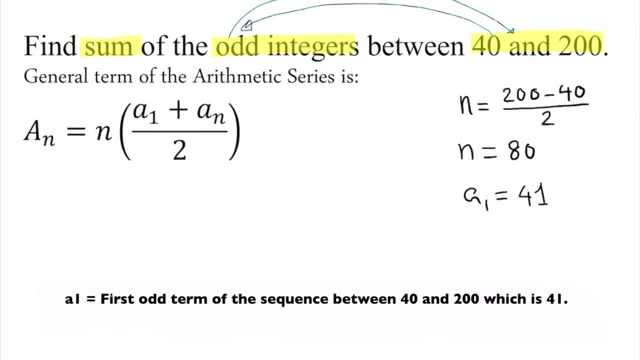 is our first odd, which is 41.. Of course we're looking for nth term, So a sub n is equal to. this is the last one, But before the last one, which one is the odd? So odd is 199.. One less. 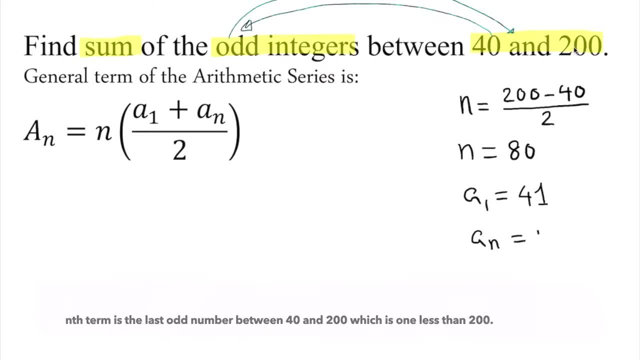 hundred, which is 199.. So 199.. So we have everything That's highlighted here, actually what we have so far. So we have the n, we have an, we have, sorry, down here an And we're going to substitute everything right in the problem here right now. formula: So n is 80,. open parentheses a1,. 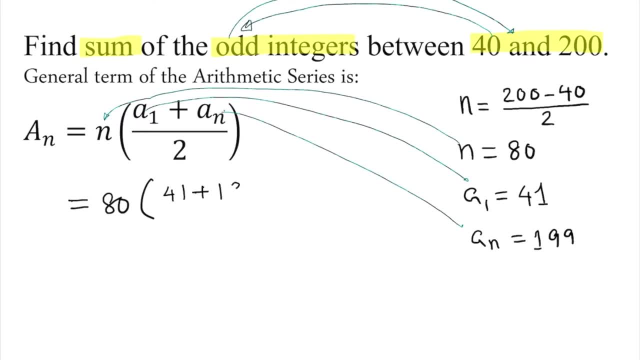 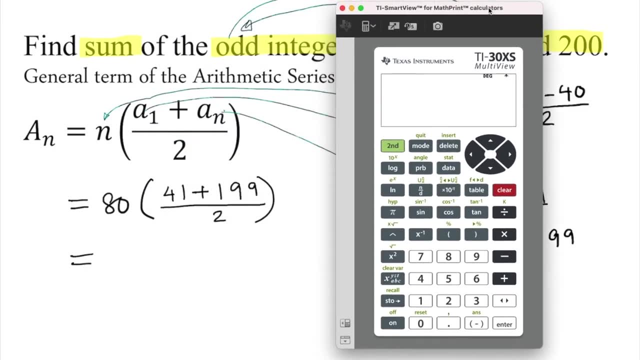 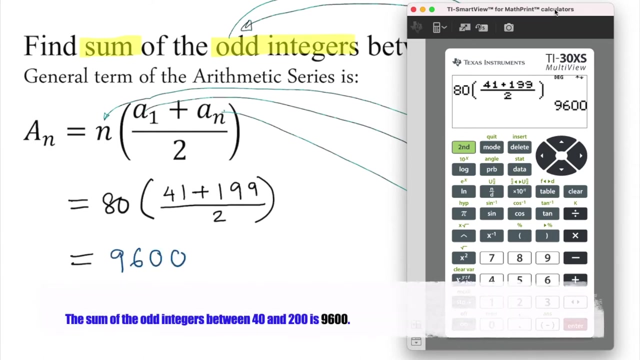 which is 41 plus 199, 199 over 2 close parentheses. so we have everything. so we're just gonna plug it in here. so we have 80 open parentheses. press n over d, 41 plus 199 over 2 to the right close parentheses. enter so 9600, beautiful. so we have 9600, 9600. what is that? 9600, 96, that many.